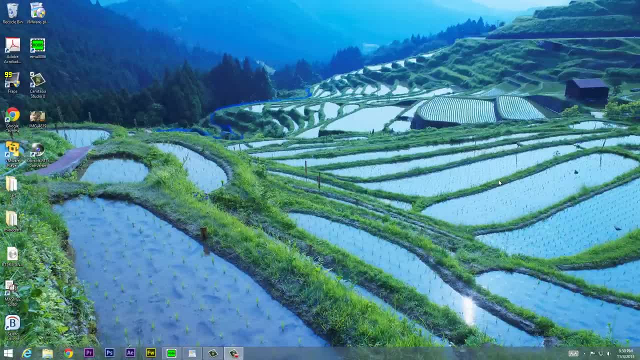 What's up guys? I'm Arsene from RossMirrorTechcom and this is another tutorial in assembly programming. Now, in this class, I'm going to talk about the push and the pop instructions, so let's get started. Let me first start off by saying: normally, when we move a value from one area into memory, 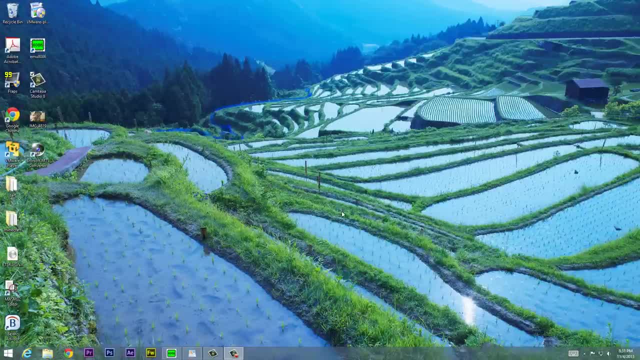 we have to specify the exact address. The program would have to specify the exact address in memory right, Which takes up time, it slows down the CPU and it's just really inefficient altogether. But assembly programming, they figured out a way around this. 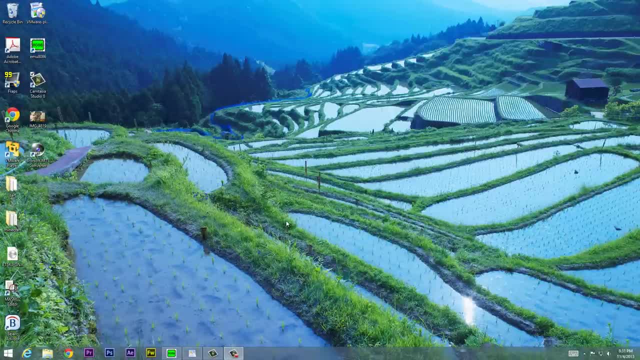 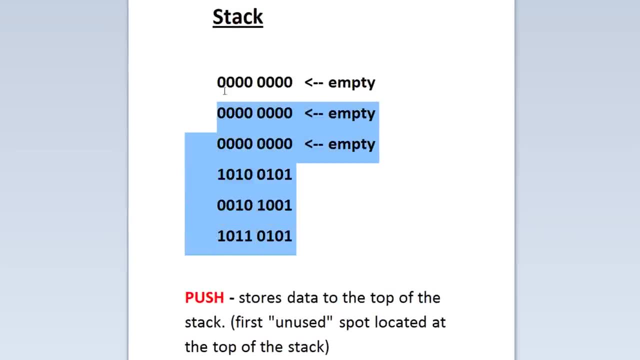 Now they figured out a neat technique which they call push and pop, so you don't have to write those addresses. So let me show you exactly what push and pop do. Now, over here I have a stack- right, This is a memory stack. 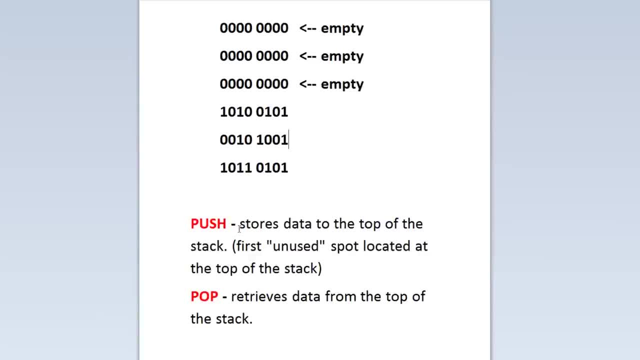 Let's first talk about push, Push. when we use the push instruction, it stores the data on the top of the stack. It goes all the way on the top and it looks for the first unused memory address on the top of the stack. 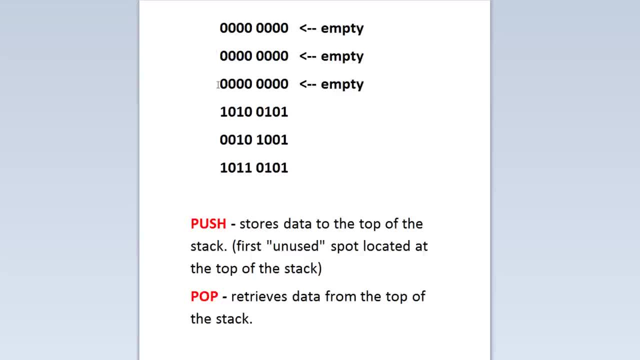 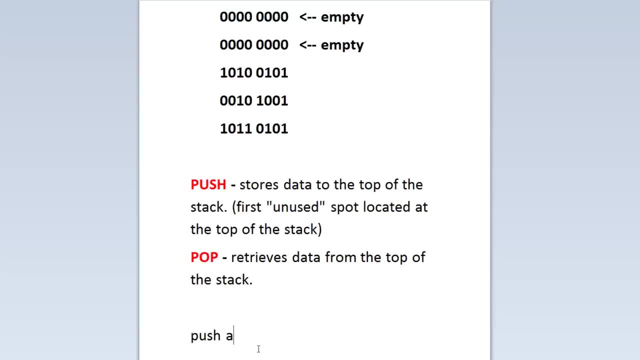 So it'll go all the way on the top and look for the first empty spot, which would be this: Let's say I use the push instruction right now, Let's say I push AX right, And let's say AX had the value of: let's say, 1, 2, 3, 4 space: 1,, 2,, 3, 4.. 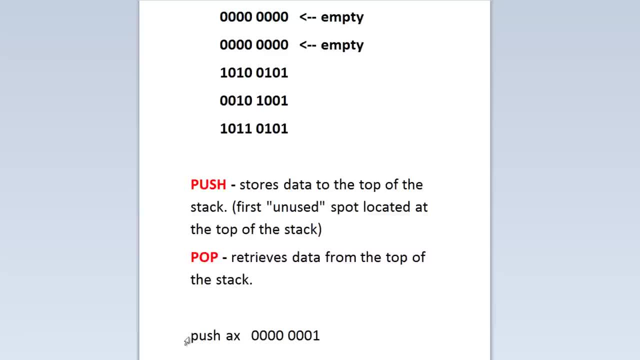 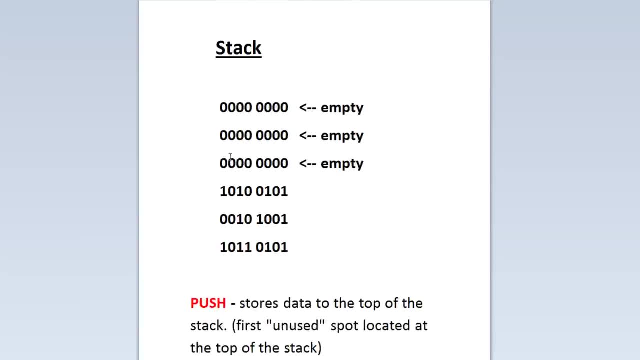 I'm sorry. 1, 2,, 3, 1, had the value of 1, right. once I could push AX, it's going to take this value right And it's automatically going to copy it to the first empty namespace there. 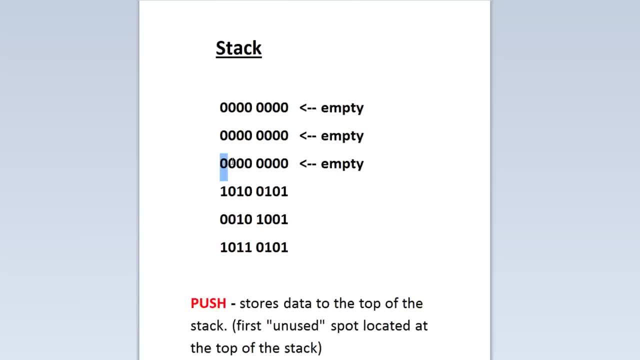 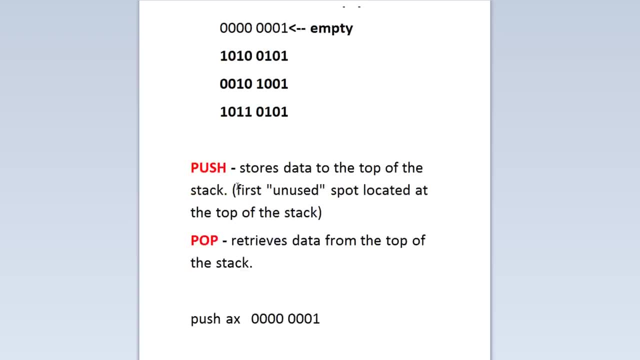 And it's automatically going to copy it to the first empty namespace there spot on the top of the stack. this would be the first empty spot on the top of the stack, so it would paste it here, right. so every time we push, it copies data on the top and it looks for the first. 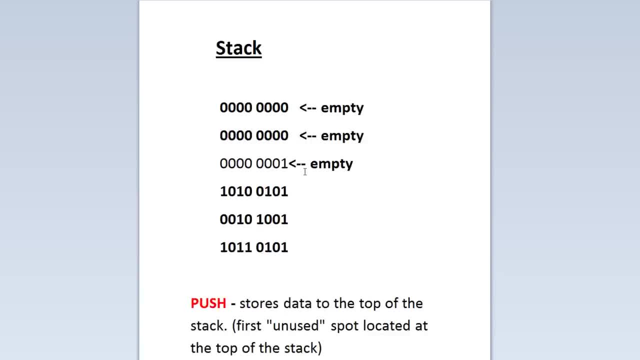 empty spot. so the reason why this is more efficient. again, let's say, when we're moving memory in a program, normally we have to specify exactly what that address and the size and everything, and that that takes up time. that's it. there's more lines of programming you have to write and it. 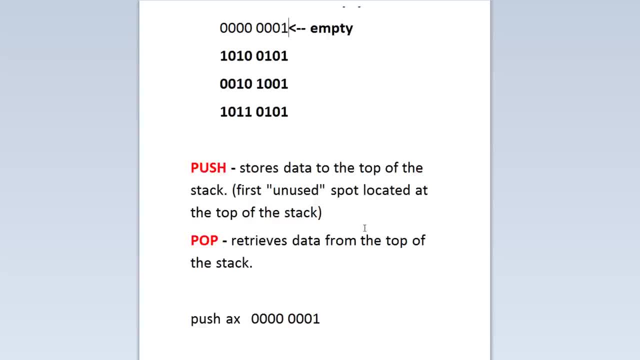 slows the program down. so that's why we use the push instruction. but now let's talk about the pop instruction. now the pop instruction retrieves data from the top of the stack. so let's say I used pop ax right now push ax it. whatever values in ax again was gonna, it's gonna be saved in the first. 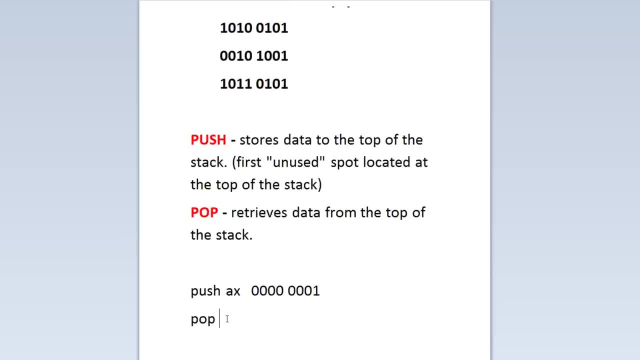 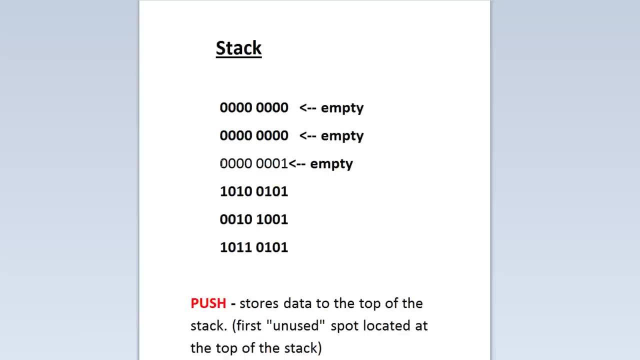 unused spot on the top of the stack and it's going to be saved in the first unused spot on the top of the stack. let's say I pop CX now pop goes all the way on the top and it's gonna look for the first pushed or the last pushed spot, so this would be the last push spot. it takes this and it copies. 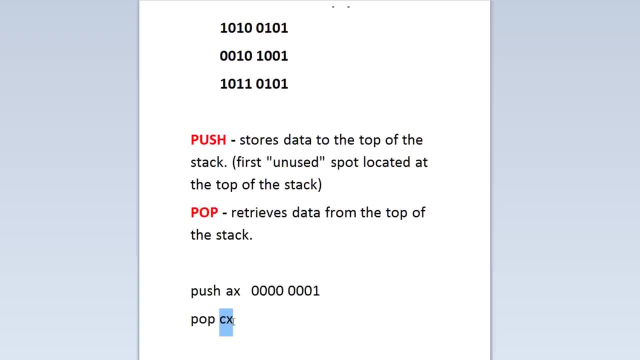 it right and it'll copy it straight into CX. so that's what pop does. pop retrieves the data from the top of the stack, basically. so there's no need to specify exact addresses, and it's just really simple to do if you want to just give you use as a placeholder. 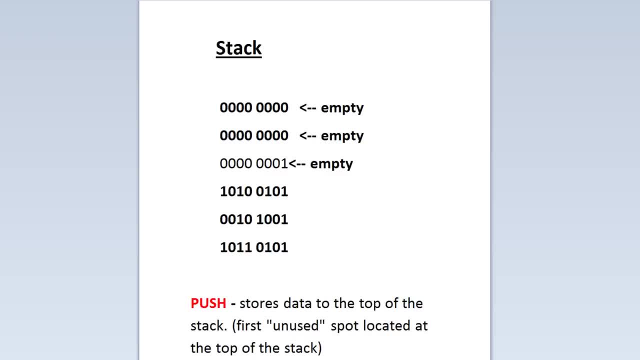 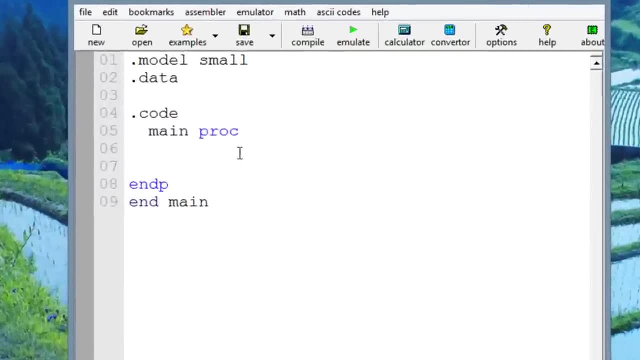 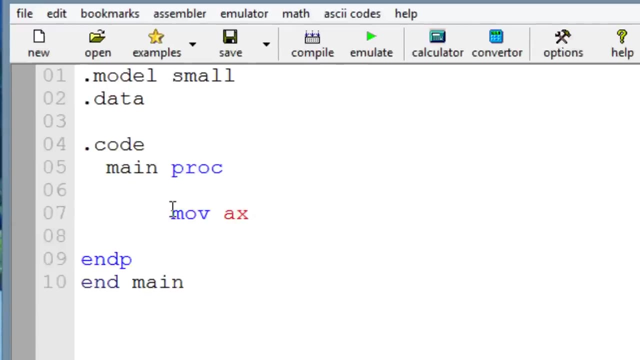 and it's really simple to do so. let me demonstrate this in a program. let's open up MU 8086 here now. first thing I want to do is I want to use the ax register and I want to give a value to the ax register. so I'm going to move into ax the value of one right, so the ax register has a. 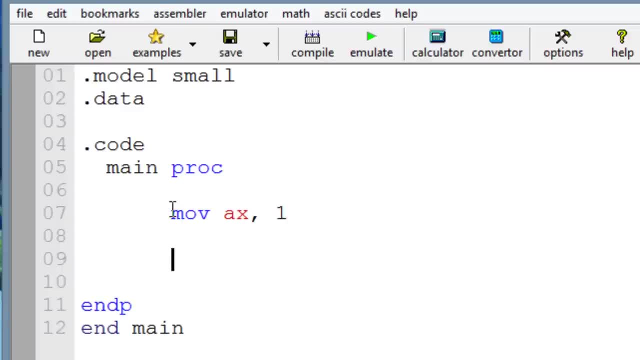 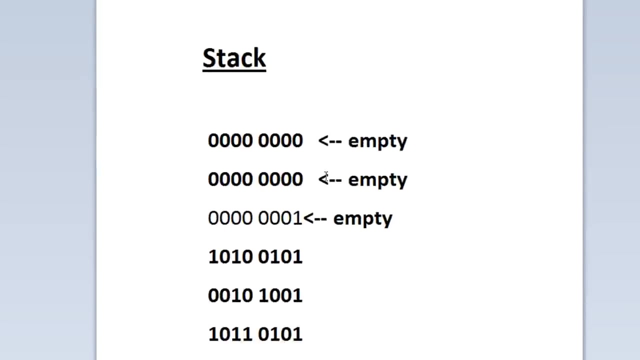 value of one. now I'm going to pop, I'm sorry. now I'm going to push ax. okay, again, ax has a value of one, right. once we use the push instruction ax, it's automatically gonna be copied to somewhere on top of a memory stack that's empty. so let's say this would be the. 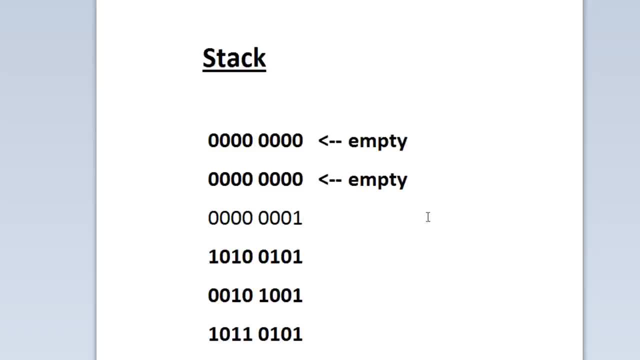 next we just use this one, right? so let's say: this would be the next empty spot. it would copy that and I'm pasted onto here. that's all. that's all it is. so let's go back to MU 8086. so now let's say: 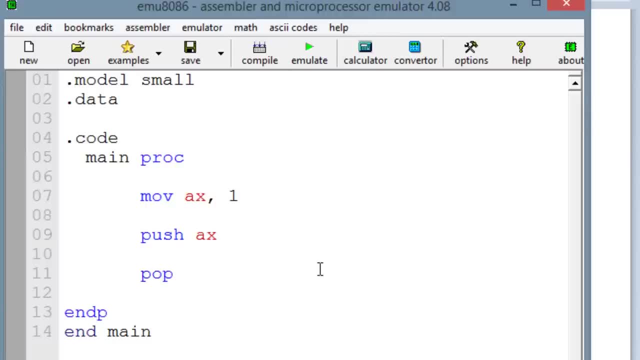 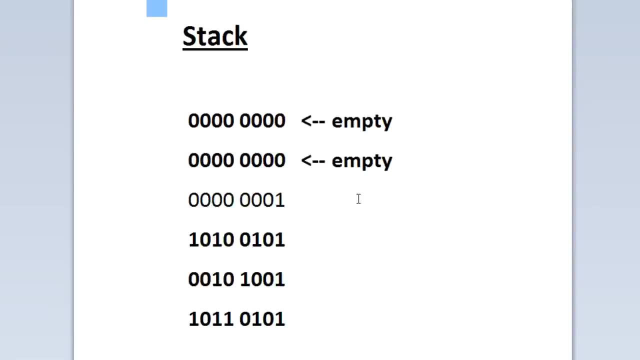 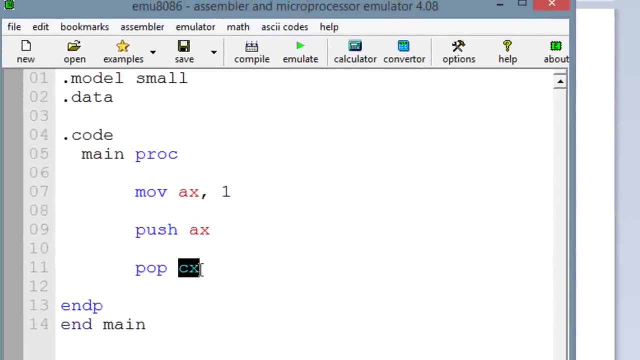 we pop. now we want to pop CX again. pop retrieves data from the top of the stack, so once we pop, it's going to jump to the next spot that was used, the last push point. basically, it copies that and it stores it into the, the destination right, which would be here right. and now let's hit.